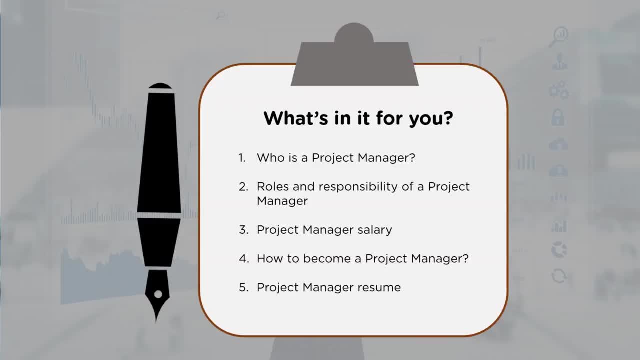 check the roles and responsibilities of a project manager. Moving forth, we will analyze the salary of a project manager and the steps that will help us become a project manager. Finally, we will see a project manager's resume. So, without any further ado, let's get started. 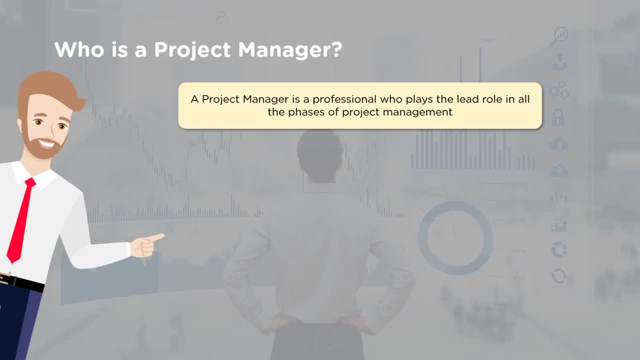 with who is a project manager. Project manager, in simple words, is a professional who manages the project. Project manager plays an integral role from the first phase of the project life cycle to the last phase of project life cycle. This individual is a part of all the activities. 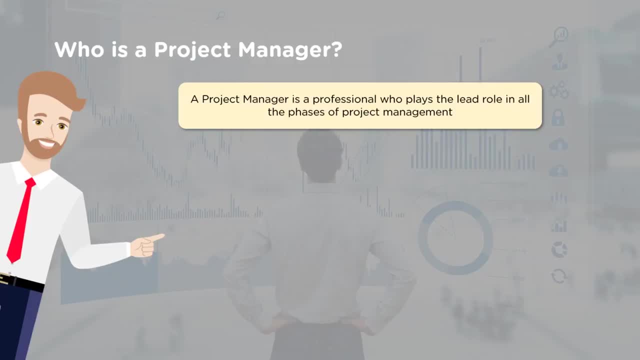 that produce the final deliverables and strive towards the success of the project. Now let's consider some must-have skills of a project manager. First we have is strong communication skills. The communication skills help the project manager to communicate the organization's mission and vision to the team members in a clear, concise manner. These 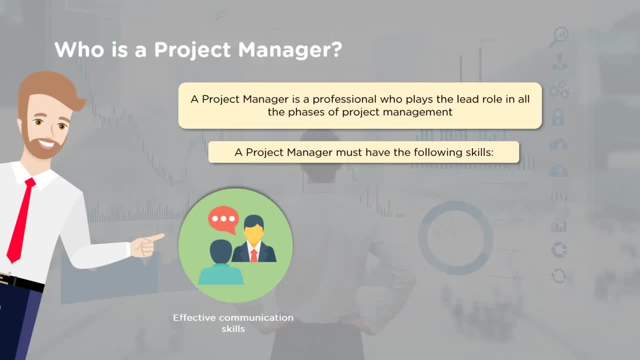 communication skills help project manager to explain their thoughts and requirements to customers and stakeholders. The next we have is effective leadership skills. that helps in forming a team of skilled professionals and lead them in the best possible manner. The next skill that a project manager must have is a strong communication skills. These 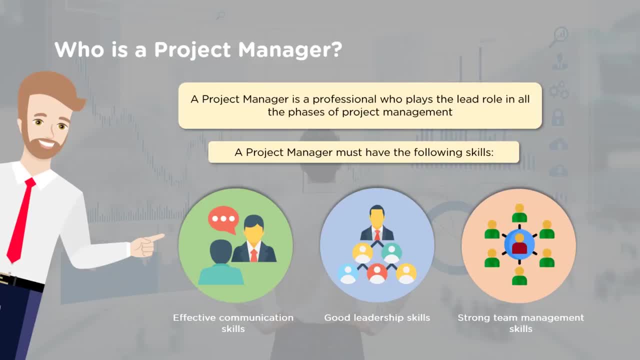 a project manager must have is a team management skill. As a project manager, it is very important to know how to manage your team to achieve a common goal with complete harmony. A project manager must have strong negotiation skills, as project managers have to negotiate. 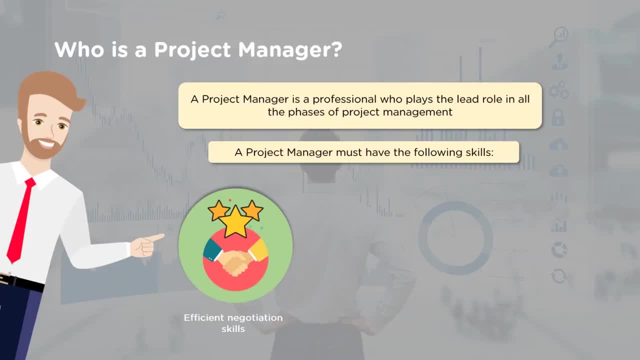 at each and every step. This negotiation might be with the customers, stakeholders or team members. These negotiation skills become of utmost importance when project members get into a fight or an argument. Then we have critical thinking. This is what makes a project manager more effective and efficient in project management. 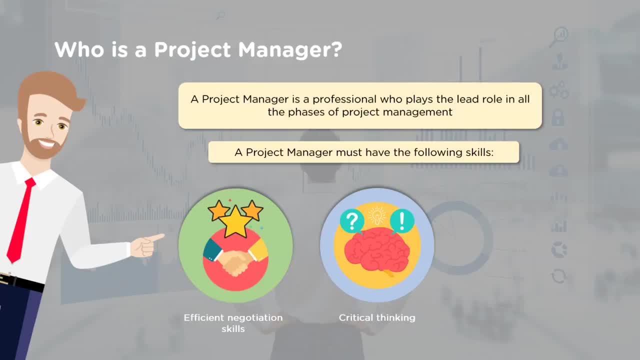 This thinking capability is needed to take difficult steps, talk to stakeholders and resolve several issues throughout the course of the project. The last skill that a project manager must have is risk management skill. Handling a project is an important step, But what is equally important is risk management. 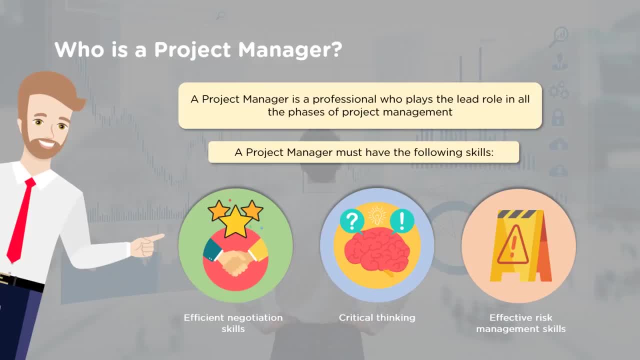 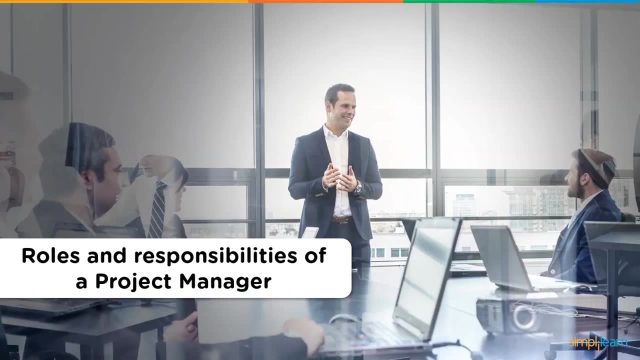 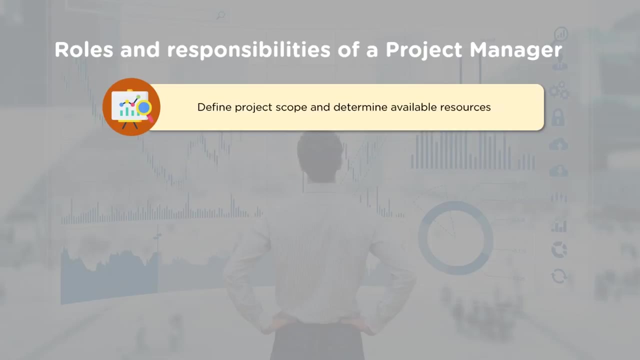 This is the process required to identify, analyze and respond to the risk factors throughout the project lifecycle. Now, when we know who a project manager is, we must have a look at the roles and responsibilities of a project manager. The first and the foremost role of a project manager is to set up a project scope check. 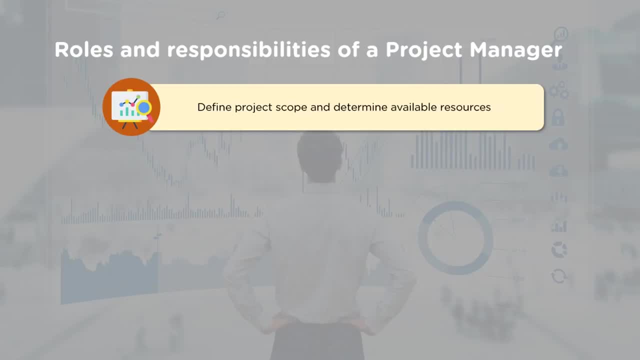 its feasibility and determine the resources that are needed to satisfy the project scope. Second role that a project manager has is the development of a project plan according to the project scope. The plan is needed to encourage the team to hard work with all their dedication. 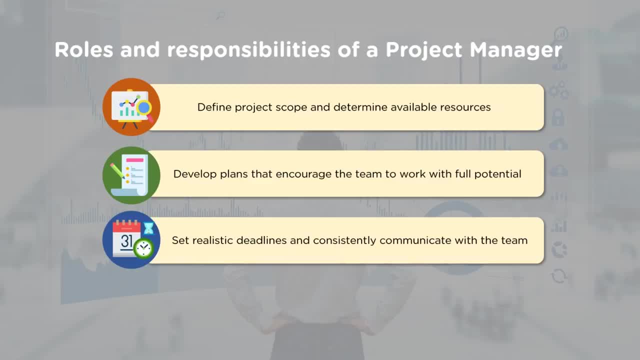 Next, a project manager is responsible for the development of a project plan. The project manager is responsible for the development of a project plan. He or she is supposed to set deadlines for the project deliverables. He or she is supposed to manage time as a priority and communicate with the team at 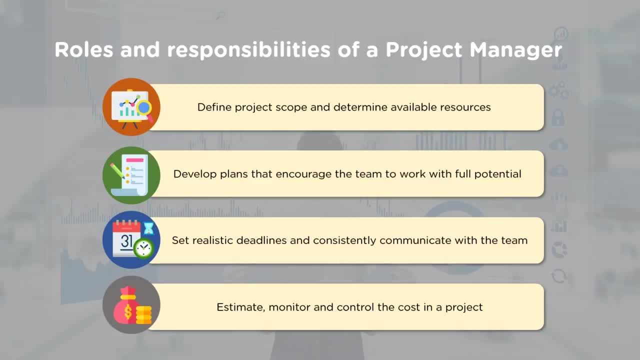 regular intervals. Next important role is to analyze, track and control the budget of the project. Project manager has to make sure that the project does not run out of budget and is optimized as possible. Moving forth effective communication is one of the most important skills of a project. 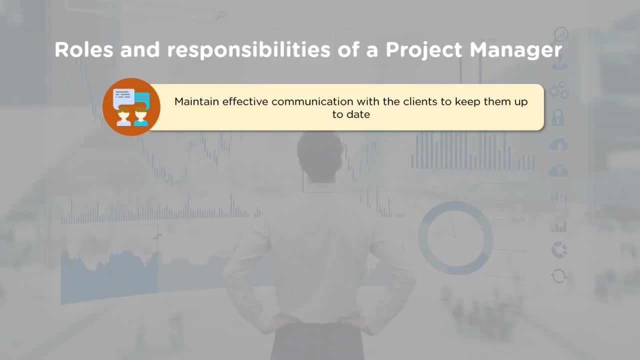 manager. He or she is supposed to maintain communication with all the stakeholders who are involved. He or she has to make sure that it alone establishes a powerful communication model that also bases arms on the task and also creates dynamic interaction amongst the stakeholders. Then we have is the identification and evaluation of the risk in a project. 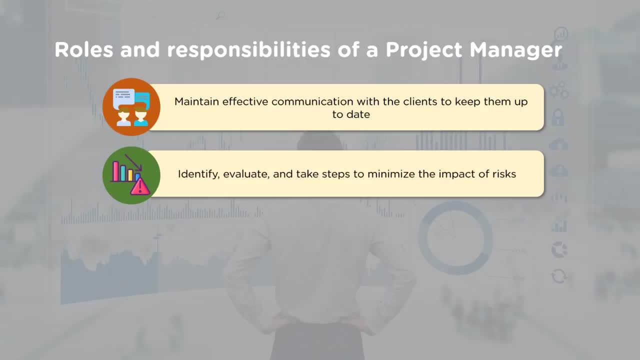 Project manager than we have is. we should take steps to minimize the effect of risk in a project. The next role of a project manager is to track and control the performance of the team. This assist in yielding the best output with the least number of resources. 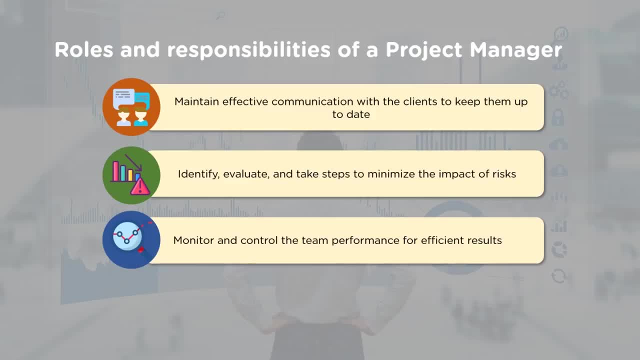 The next role must take steps to minimize the effect of risk. The next role is to always control and control the position of a team. The project manager must provide information and documentation of all the steps involved in project managing. Then we have is the identification and evaluation of risk in a project. 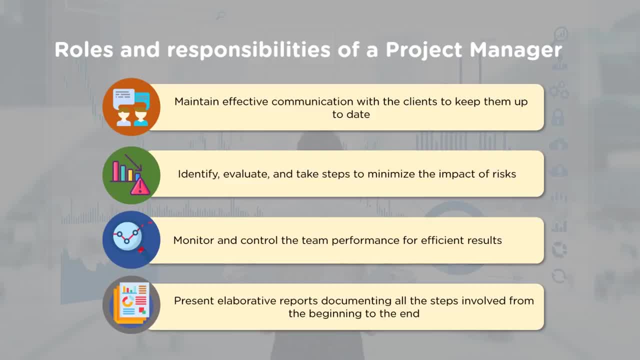 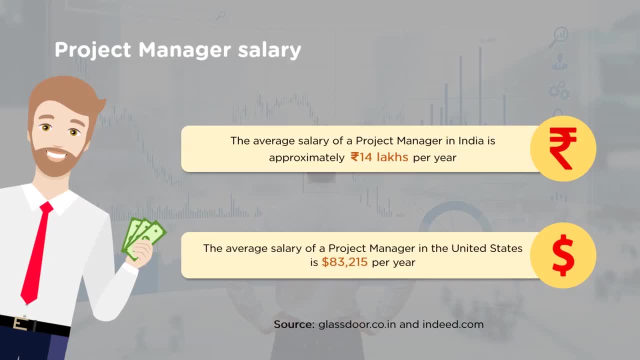 that happened in the project will not happen again in ongoing projects. Now it's time for us to check the salary of a project manager. The data shows that an average salary of a project manager in India is approximately 14 lakh rupees per annum, while the average salary of a project manager in 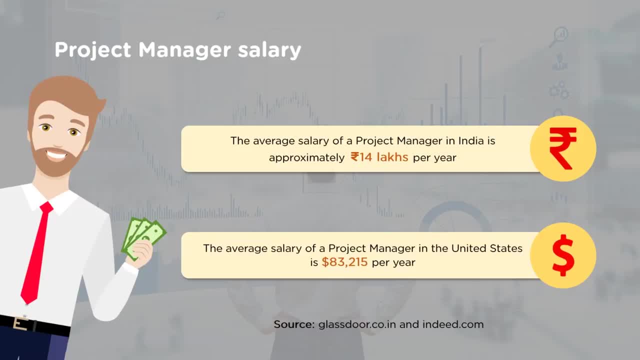 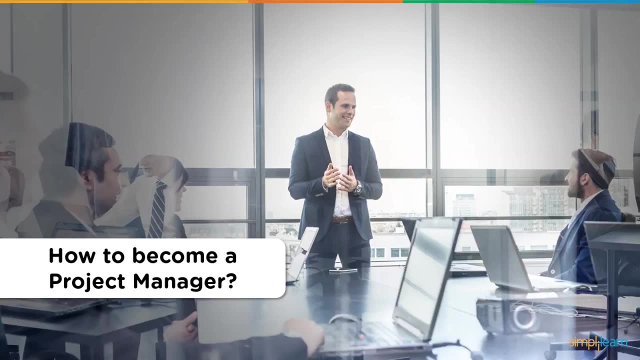 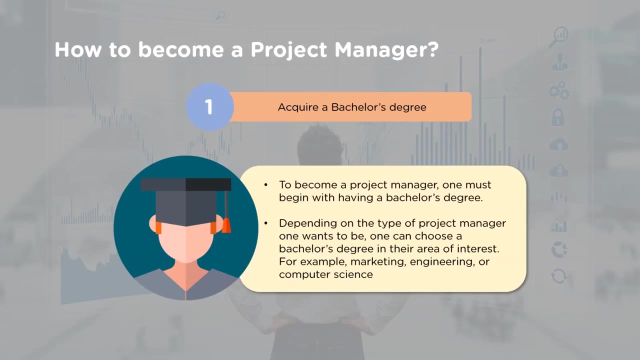 United States is 83,215 dollars per year. The next important thing we must learn is how can we get a project manager's job? There are four important steps that one must fulfill to become a project manager. The first step is to have a bachelor's degree. It is important for a person to be a 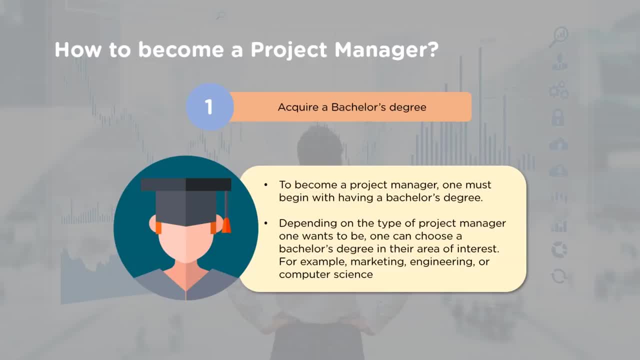 graduate. One can hold a bachelor's degree in any area of interest, like marketing, computer science or even engineering. This entirely depends on the type of project manager one wants to be. The second important step is gaining project management experience. This means that a person must have 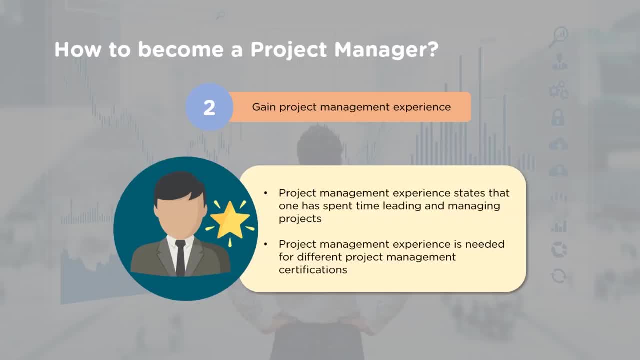 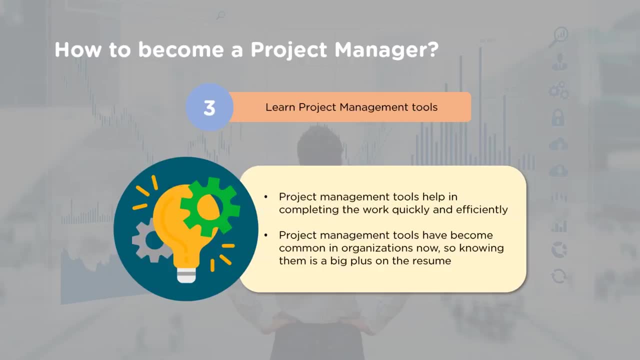 experience in leading and directing projects. Project management experience helps in taking different project management certifications, which further help in having a good paying job. The third essential step is to learn project management tools. There are different project management tools for different areas of interest. These tools help in: 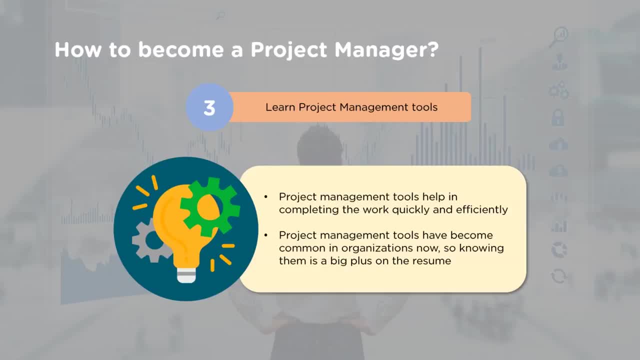 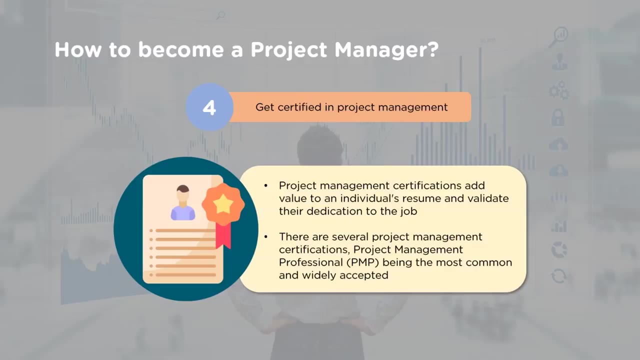 quick and efficient management of work. Project management tools are used widely by organizations. now, Learning these tools will increase the chances of getting selected in one of those organizations. The fourth and the last step is getting project management certified. Project management certifications helps an individual to increase their certification. 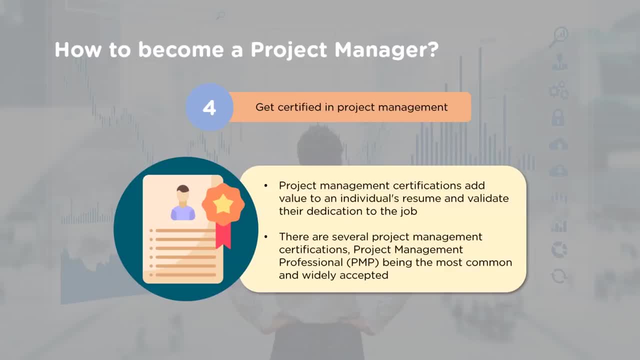 and validates their dedication to the job. Nowadays, several organizations have made it compulsory for a project manager to be project management certified. There may be several project management certifications, out of which project management professional certification, or PMP certification, is one of the most common, widely accepted certifications. The project 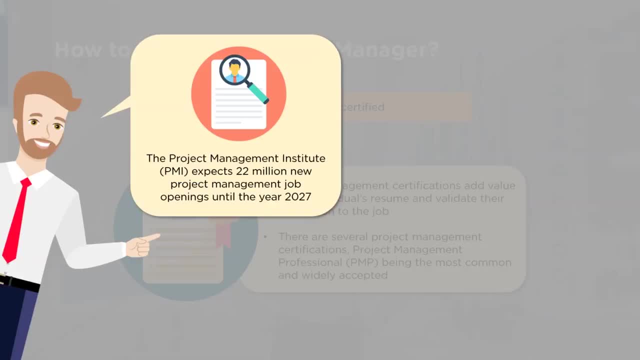 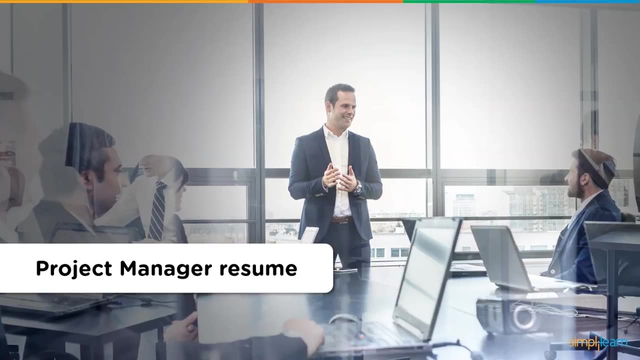 management institute, or the PMI, predicts that about 10% of officers of employment would be certified with project management certification in the form of a project management certificate. there will be 22 million new project management jobs by the year 2027. now it's time for us to know. 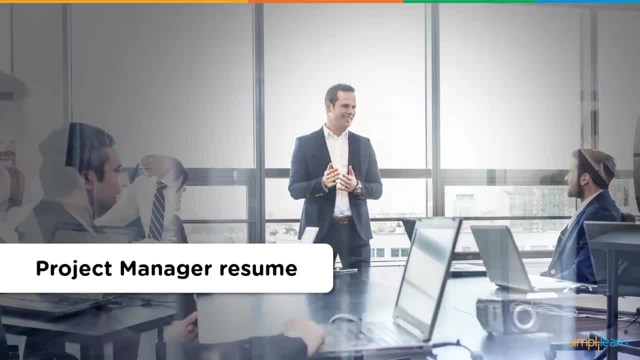 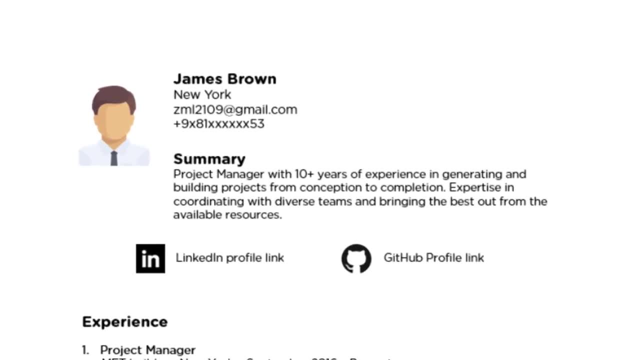 how a resume of an aspiring project manager looks like. if you are somebody looking for a project manager role or a senior project manager role, then your resume should look something like this: the summary in the beginning would include how much experience you have and anything that supports your claim of being a project manager. like here james brown has written: he has more than 10 years. 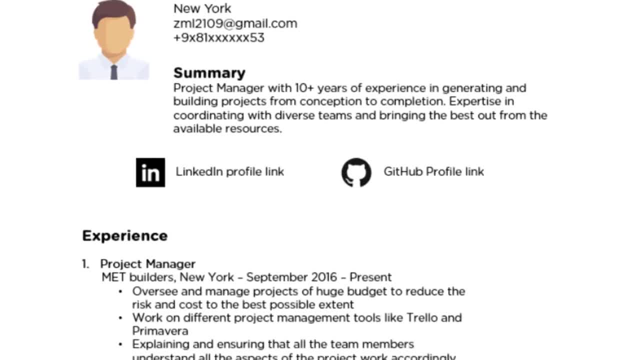 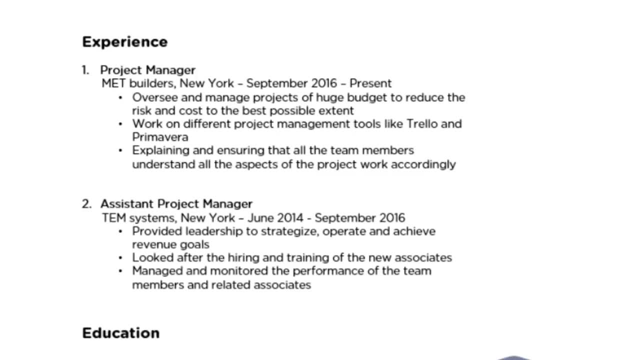 of experience with generating and building projects, then when you talk about your experience, you should put something that emphasizes on the responsibilities that you had in your area of expertise. put something that shows your skill set for the desired post and also something that you learned from your former job role. this shows that you have command.